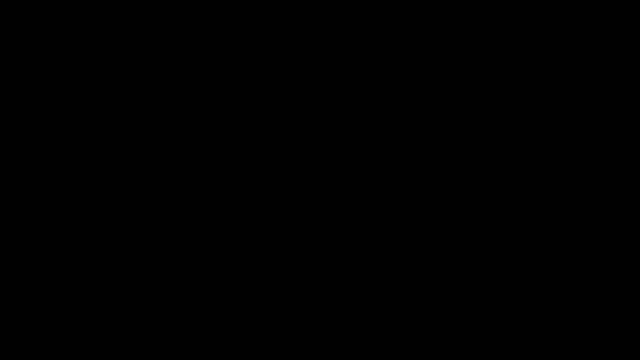 In this video we're going to focus on Bayes' theorem, But first let's go over some formulas, particularly with conditional probability. The probability of event A occurring given that event B has already occurred is the probability that event A and B will occur divided by the. 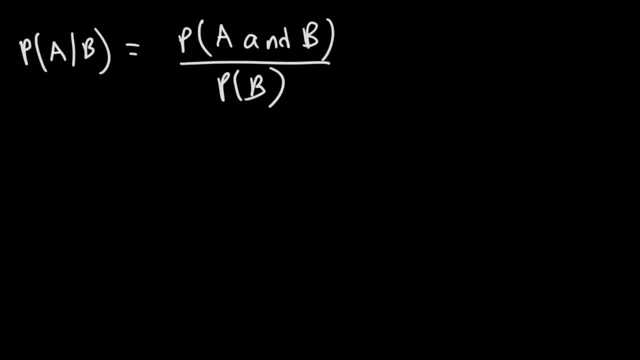 probability that event B will occur. Likewise, we can say that the probability of B given A is equal to the probability of B and A occurring divided by the probability that event A will occur. Now, the probability that event A and B will occur is equal to the probability that event B 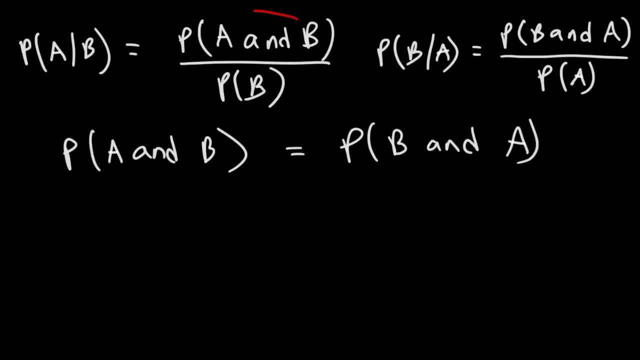 and A will occur, So. So, basically, what I'm doing is I'm setting these two equal to each other. Now, this is equal to the probability of A given B times the probability of B. So let's replace that on the left side. 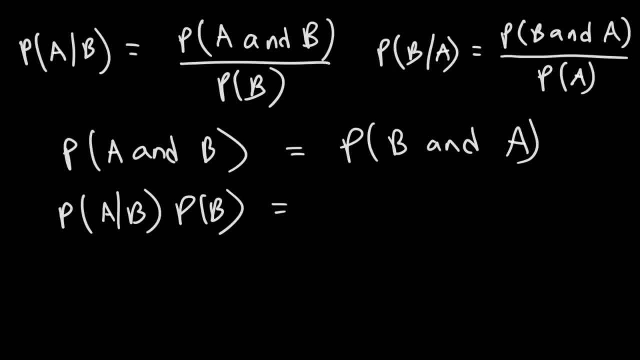 Now, on the right side, the probability of B and A occurring is the product of the probability of B occurring, given A has already occurred, times the probability of event A occurring. Now what I'm going to do is divide both sides by the probability that event B will occur. 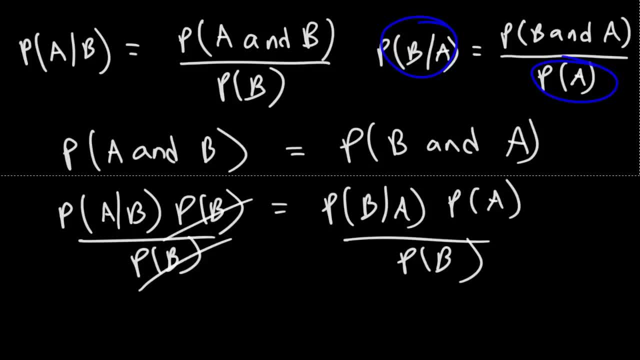 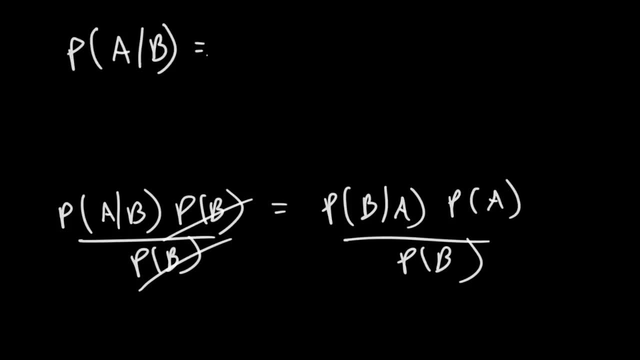 And so this is going to give me the formula that is associated with Bayes' theorem. So the probability that A will occur, given that B has already occurred, Is equal to the probability that B will occur, given that A has occurred, times the probability of event A occurring divided by the probability that event B will occur. 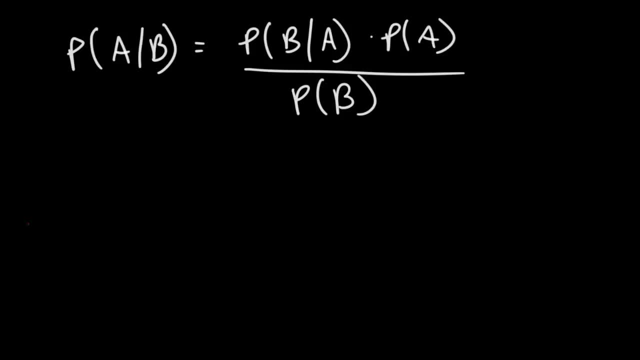 So Bayes' theorem helps us to calculate the conditional probability of an event if basically, you know the reverse conditional probability with some other probability values as well. But this is the basic formula of the Bayes' theorem. So P of A given B is equal to P of B given A times P of A divided by P of B. 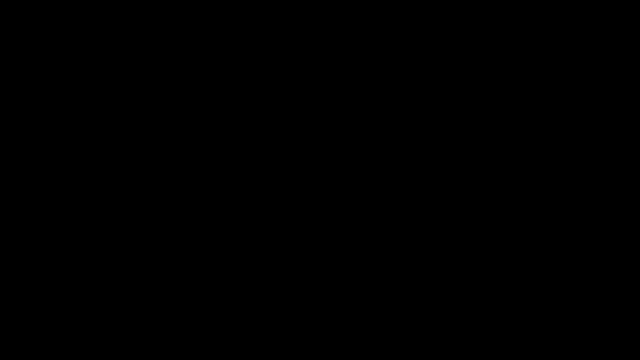 Now let's use a simple example that will illustrate the use of Bayes' theorem. So let's say that in a bottle there's a bunch of pieces of papers with numbers on it. Let's say: event A represents the following numbers being drawn: 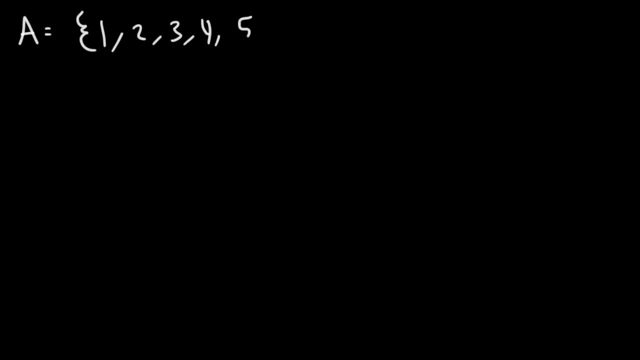 1,, 2,, 3,, 4, and 5.. Okay, Now let's say event B represents the numbers 4,, 5,, 6,, 7,, 8, and 9.. Now what is the probability of A given B? 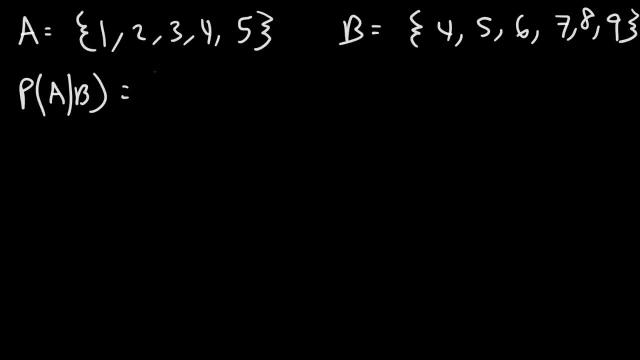 Let's use Bayes' theorem to calculate this particular probability. Even though we don't need to for educational purposes, let's do it Now. what I'm going to do is create a Venn diagram. Okay, So let's say the first circle is for event A and the second one is for B. 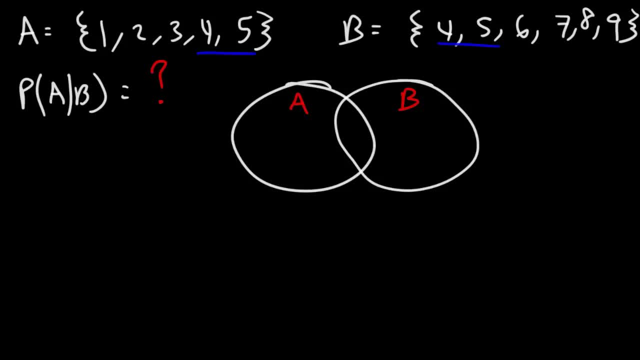 So A and B has these two numbers in common: 4 and 5.. So that's the intersection of A and B. A also has the numbers 1,, 2, and 3.. B has the numbers 6,, 7,, 8, and 9.. 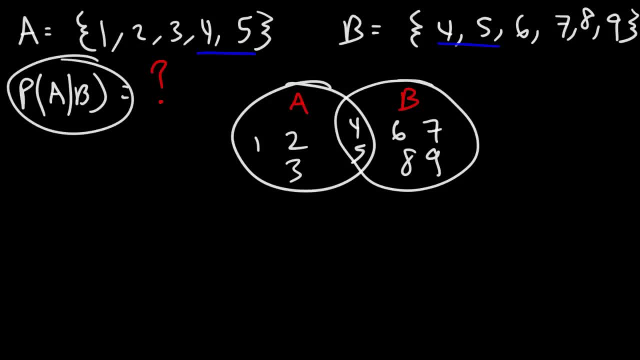 Now, in order to calculate this using Bayes' theorem, we need to know the probability of event A occurring, the probability that event B will occur and, basically, the reverse conditional probability, the probability that B will occur given that A has already occurred. 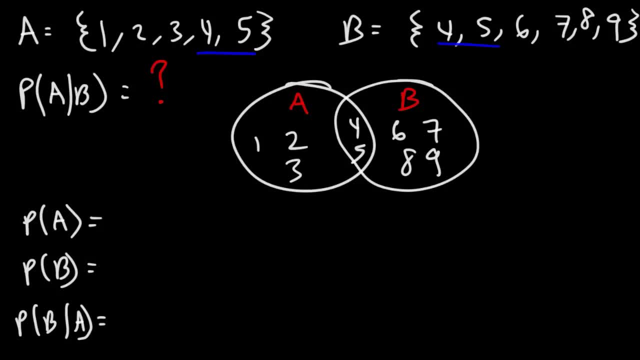 So what is the probability that A will occur? Well, we need to write the sample space. The sample space represents all of the possible numbers, The numbers in A and B. So the numbers that we can get represent all of the natural numbers from 1 to 9.. 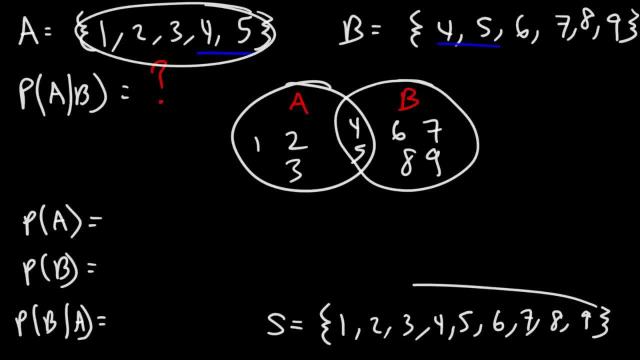 So A has 5 out of the 9 possible numbers that we can choose from. So the probability that event A will occur, assuming that each number has an equal chance of being drawn out of the bottle- is going to be 5 out of 9.. 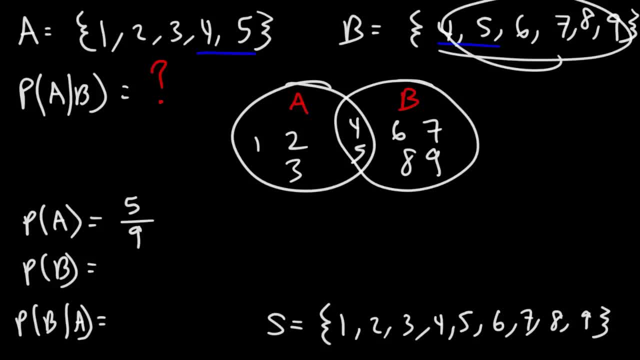 Now B has 6 numbers out of the 9 numbers here. So the probability that event B will occur is 6 out of 9.. Now what about the next one? What is the probability that B will occur, given that A has already occurred? 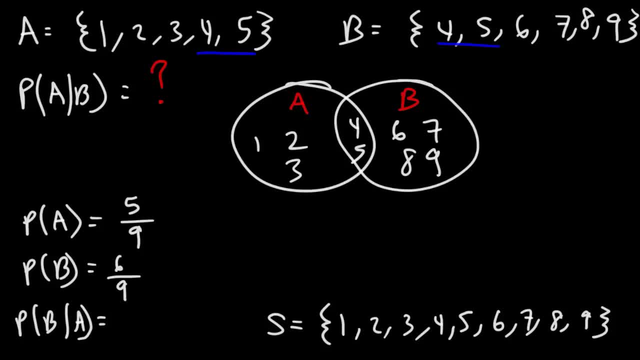 There's a formula for that which we talked about earlier in this video. But to think about it conceptually, how much of B is in A? A has 5 elements. It has the numbers 1 to 5.. Out of those 5 elements, what is B? 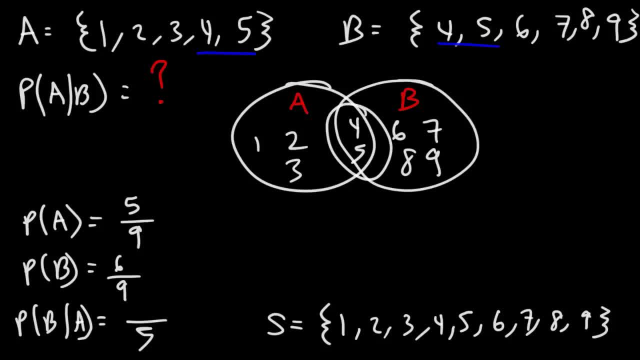 Well, A has 5 elements. Out of those 5 numbers, there's only 2 numbers. that is in B. that is part of A. So the probability that B will occur, given that event A has occurred, is 2 out of 5.. 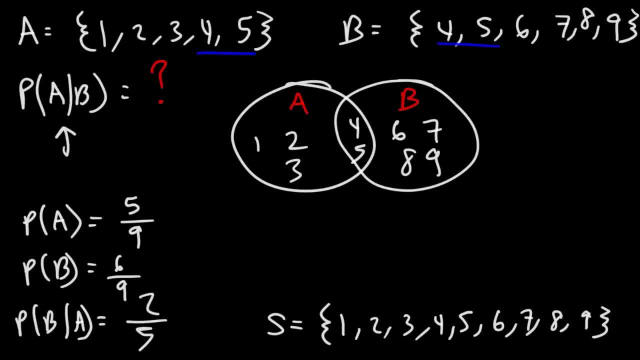 So now, with this information, we can calculate this particular conditional probability. The probability that A will occur, given that B has already occurred, is going to be P of B of A, or rather B given A. What we need to do is just add from here P of A over P of A over P of B. 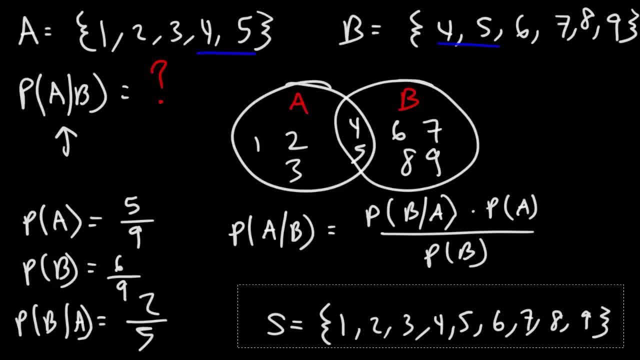 Let me get rid of this. P of B given A. that's what we have here, That's 2 over 5.. Times P of A, which is 5 over 9. Divided by P of B, which is 6 over 9.. 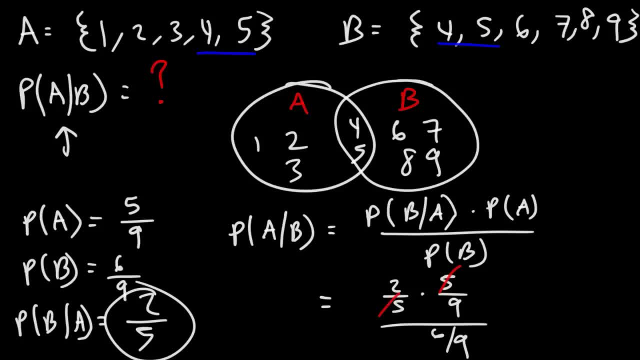 Right now we could cancel The 4 over 5. 1 over 8. P of A over P of B, 5. P of B given A, which is 2 over 9. 5. And if we multiply the top and the bottom of the fraction by nine, we can also cancel. 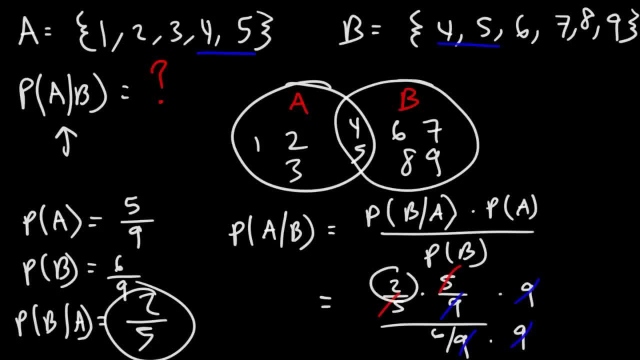 the nines. So we're left with two over six, which reduces to one over three. So the probability that A will occur, given that B has already occurred, is one out of three. Now let's confirm that using conditional probability. So P of A given B is the probability that event A and B occurs over the probability. 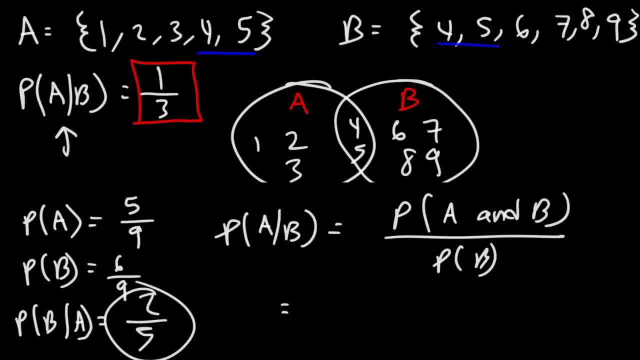 that B will occur. So we know that the sample space has nine numbers. How much of that is A and B? The intersection of A and B is basically two numbers, four and five. So the probability that event A and B will occur is two out of the nine possible numbers. 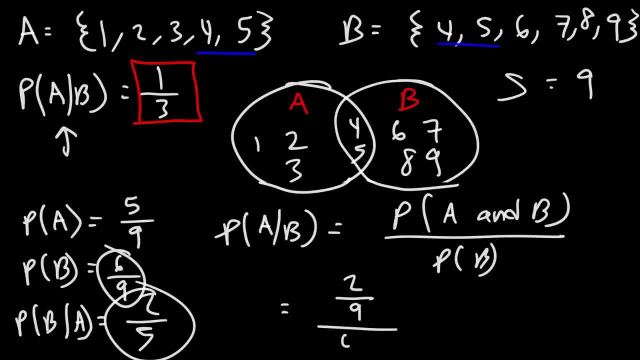 Now the probability that B will occur is what we see here. It's six over nine. So multiplying the top and the bottom numbers by nine, we're going to get the same result. Initially, it's going to be two over six, which reduces to one over three. 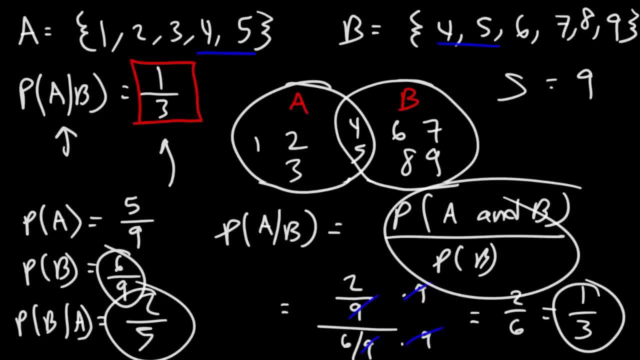 Now. granted, we could have done this from the beginning. We could have done this from the beginning. We could have done this from the beginning. But now you see how Bayes-Durham works with the formula that we wrote earlier. But let's consider another example in which we could use the Bayes-Durham formula. 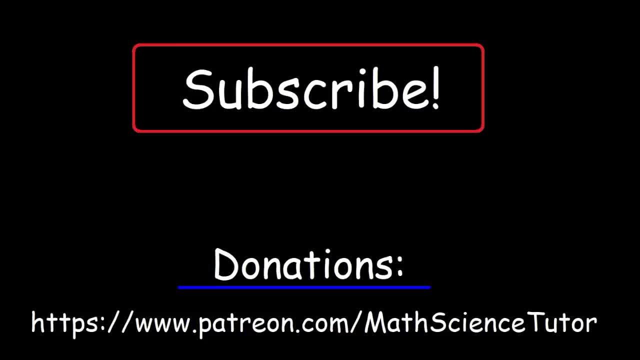 Now for those of you who truly value this video. if you want to show your appreciation, one of the best ways you can do so is by subscribing to this channel, And it really doesn't take too long. Just click on that red button at the bottom of the screen, and that's it. 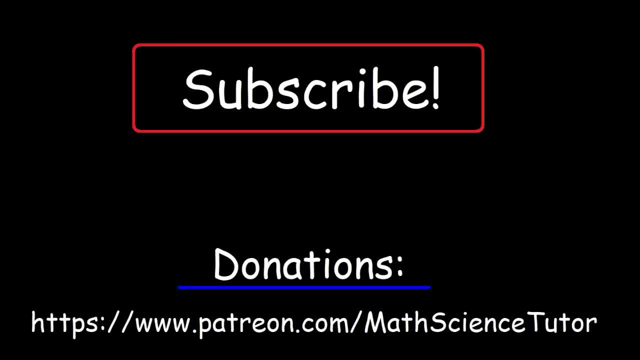 By the way, if you decide to do so, don't forget to turn on or click on that notification bell. Now, for those of you who want to support my channel, here's the link to my Patreon page. Also, when you get a chance, check out the links in the description section below this. 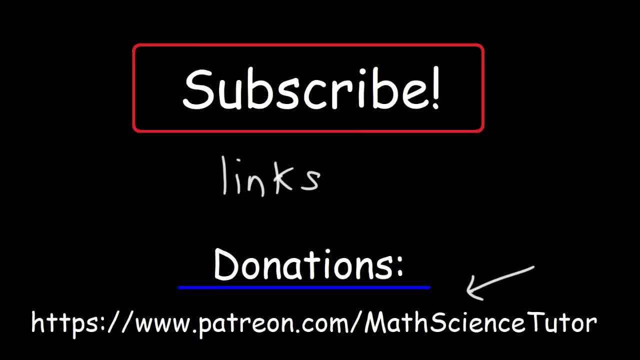 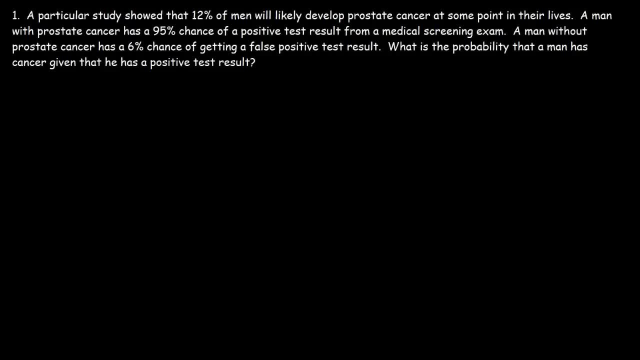 video, because I'm going to post some other resources that you might find helpful. So let's get back to the video. A particular study showed that 12% of men will likely develop prostate cancer at six. So let's get back to the video. 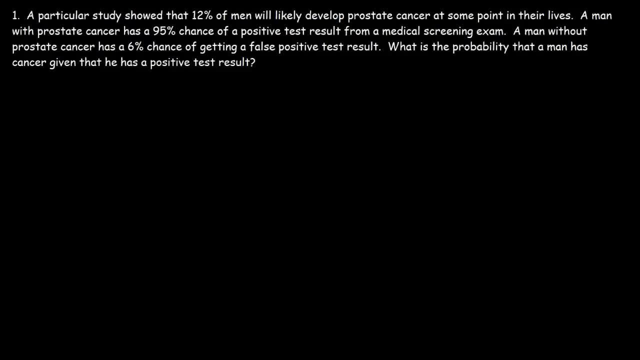 A particular study showed that 12% of men will likely develop prostate cancer at six At some point in their lives. a man with prostate cancer has a 95% chance of a positive test result from a medical screening exam. A man without prostate cancer has a 6% chance of getting a false positive test result. 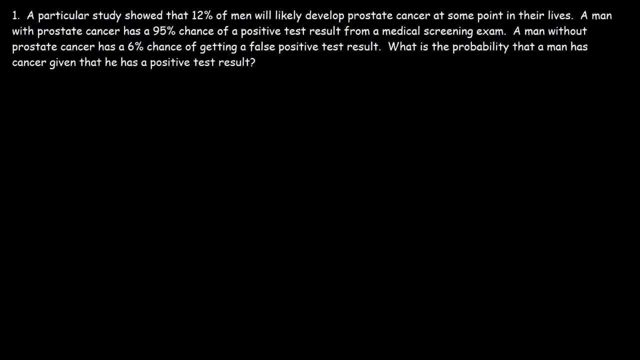 What is the probability that a man has cancer, given that he has a positive test result? What is the probability that a man with prostate cancer has a 95% chance of getting a false positive test result? What is the probability that a man with prostate cancer has a 95% chance of getting a false? 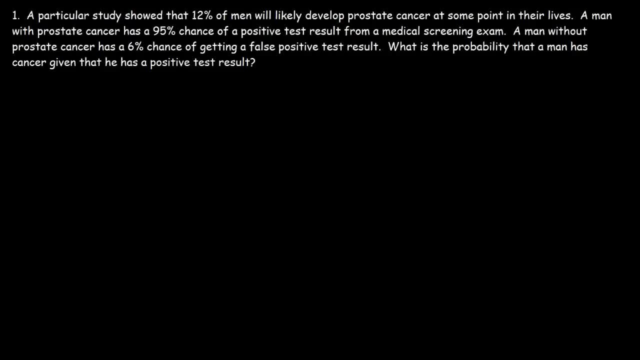 positive test result. Go ahead and try this problem. Feel free to take a minute if you need to, So let's write down what we know: The probability that a man has cancer. I'm going to write PFC- is 12%, which is .12 as. 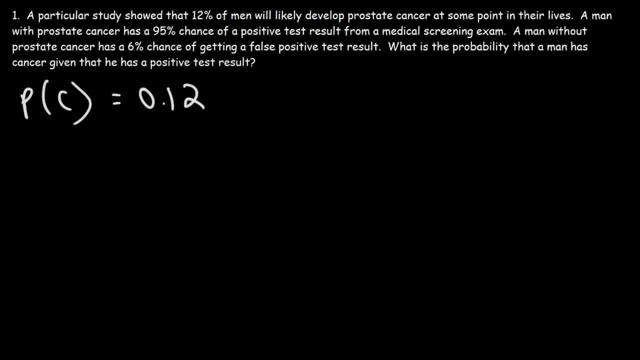 a decimal Now. the second sentence says that a man with prostate cancer has a 95% chance of a positive test result. So, given that the person has cancer, the probability that he will get a positive test result is 95% or .95.. 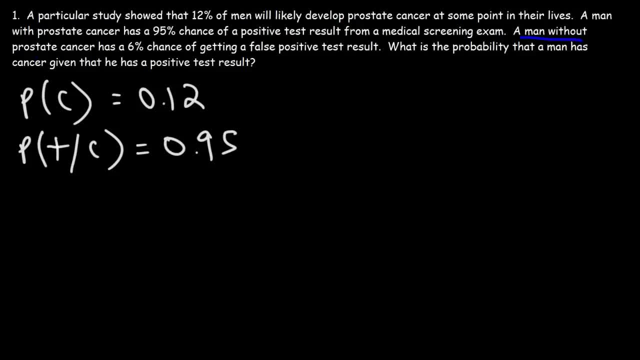 Now what about the third sentence? A man without prostate cancer has a 6% chance of getting a false positive test result. So the probability of getting a positive test result, given that the person does not have prostate cancer, is 6% or .06.. 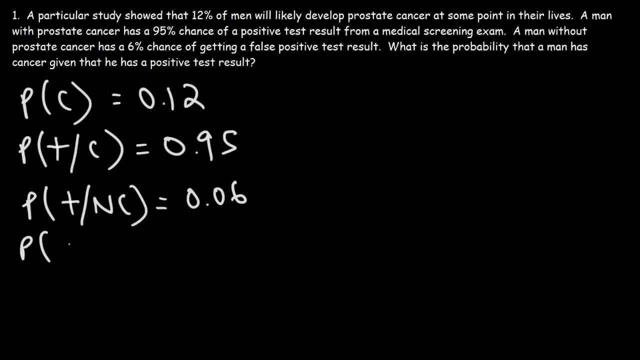 So what is the probability that the person has cancer, given that he has a positive test result? That's what we need to find. So let's write the equation for that using Bayes' theorem. So this is going to be the reverse conditional probability, which is the probability of getting. 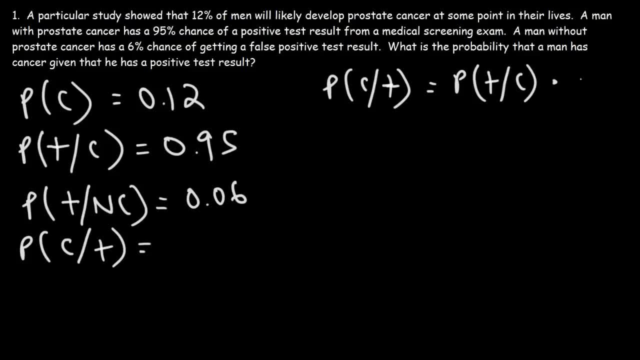 a positive test result, given that the person has cancer times the probability that the person has cancer divided by the probability that the person has a positive test result. Now, we have these two values already, but we don't have this one. How can we find it? 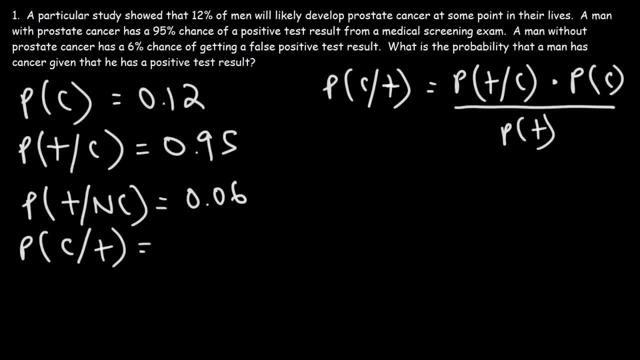 In this case it's going to be very hard, We're going to have to find it. It's very helpful to make a tree diagram. So 12% of the population will have prostate cancer. based on this particular study, That means that 88%, which is 100 minus 12 or .88, will not have cancer. 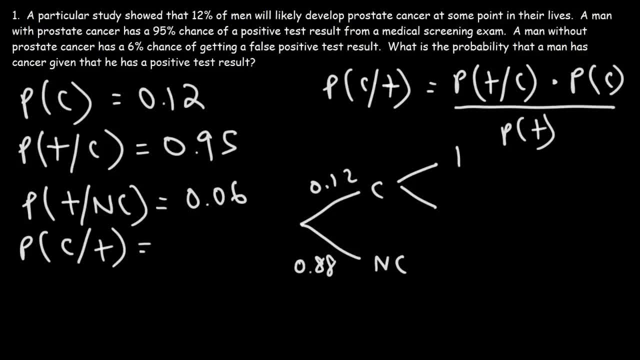 Now, out of those who have cancer, 95% of them will have a positive test result, Which means the other 5% will have a negative test result. Now, out of those who do not have cancer, 6% will have a positive test result, which means 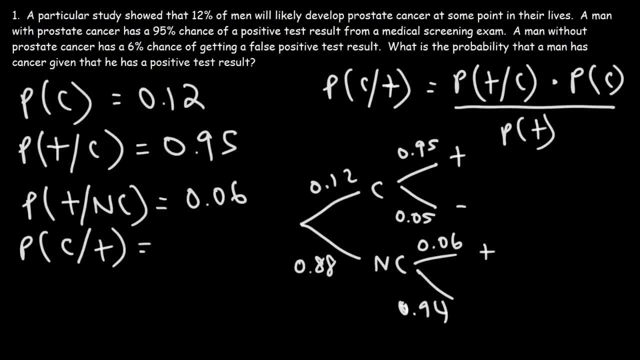 the other 94% will have a negative test result. So, using this tree diagram, how can we determine the probability that the person will have a positive test result? The probability that a person will have a positive test result depends on two events. That is, the probability that the person has cancer and they will have a positive test. 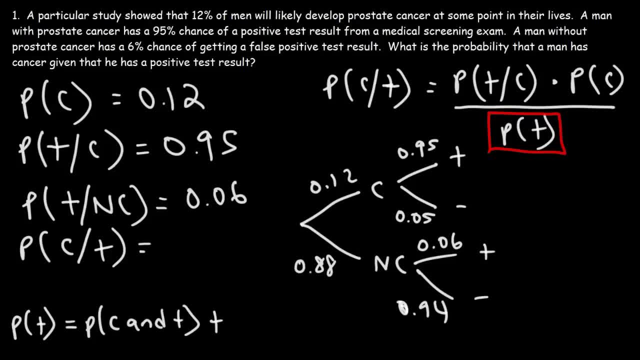 result, Or which will be represented by the addition symbol, The probability that the person does not have cancer and has a positive test result. Those are two options. Okay, cancer and has a positive test result is the product of these two values, where. 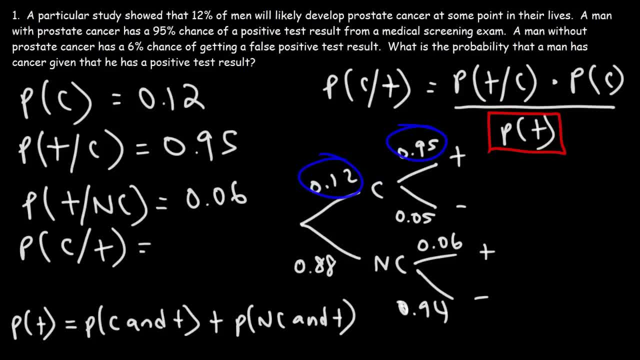 they will have cancer and have a positive test result. so it's basically 0.12 times 0.95. the probability that the person does not have cancer and has a positive test result is the product of these two values, so it's 0.88 times 0.06. 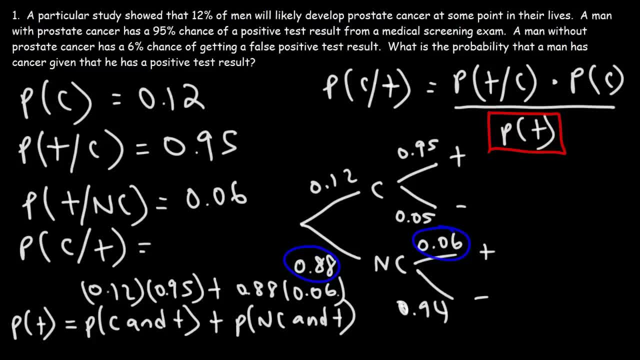 0.12 times 0.95 plus 0.88 times 0.06, that's equal to 0.1668. now I'm running out of space, so I'm going to have to delete a few things. hopefully you wrote that down because I'm going to refer to it later, if not. 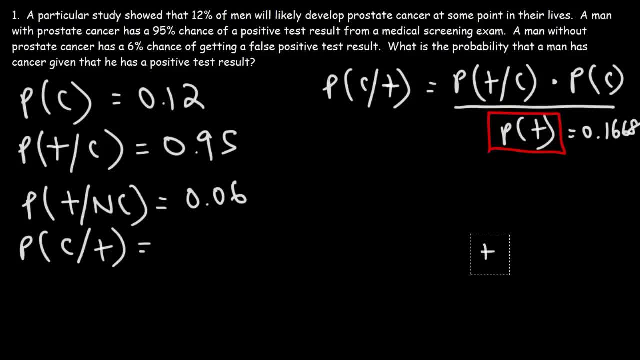 you can always rewind the video now. let's plug in the numbers into this formula. so the probability of getting a positive test, given that the person has cancer, that's 0.95. the probability that the person has prostate cancer is 12% and the probability that the man, or a man will have a positive test result is going to. 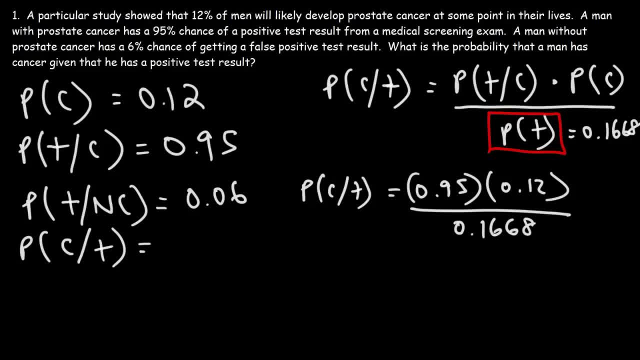 be 0.1668 or 16.68%, so it's 0.95 times 0.12 divided by 0.1668, and so you should get 0.95 times 0.12 divided by 0.1668, and so you should get 0.95 times 0.12 divided by 0.1668, and so you should get: 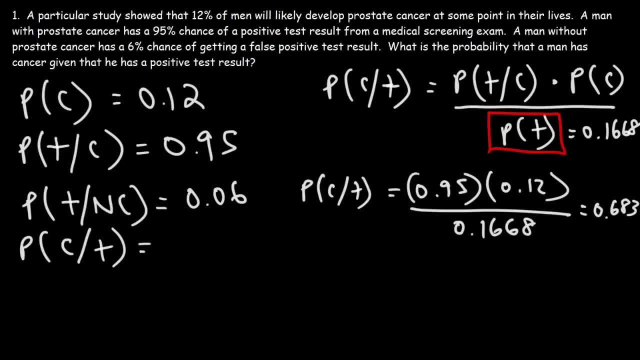 0.. casting number is 0.68345. so there's approximately a 68.3% chance that the so there's approximately a 68.3% chance that the the person will have cancer, given that they have a positive test result. so what? 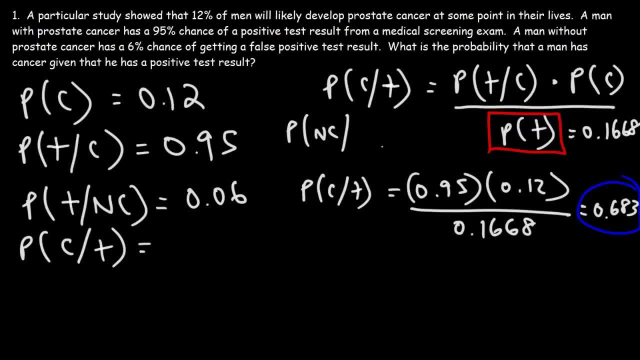 has the probability that the person does not have cancer, even though they have a positive test result. that's going to be 100 minus this number, that is, 100%, my minus 68.3%, or 1 minus 0.683, which is 0.317.. So there's approximately a 31.7% chance. 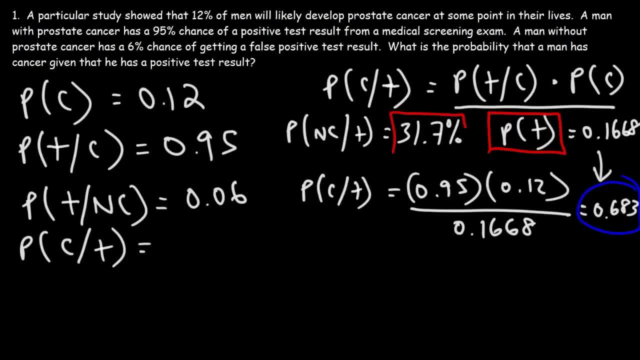 that, even though the person has a positive test result, that they do not have cancer. So sometimes, even if you get a positive test result, it doesn't mean that you have that condition. There's always a risk factor, But the answer that we're looking for in this problem 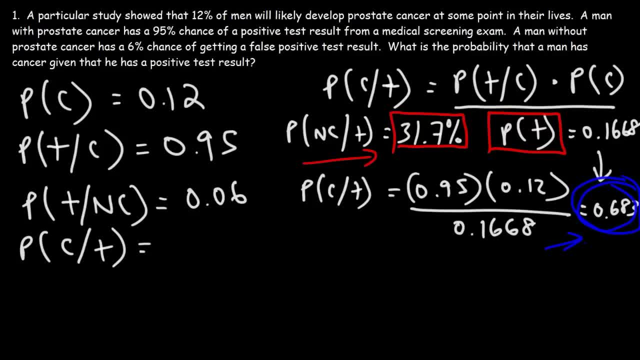 is this number 68.3%? Now, there's another way in which we can get that answer. Let's talk about how we can do it. So let's say that there's 10,000 people in a city And, based on a survey, 12% of those individuals have cancer. So we're going to use the same 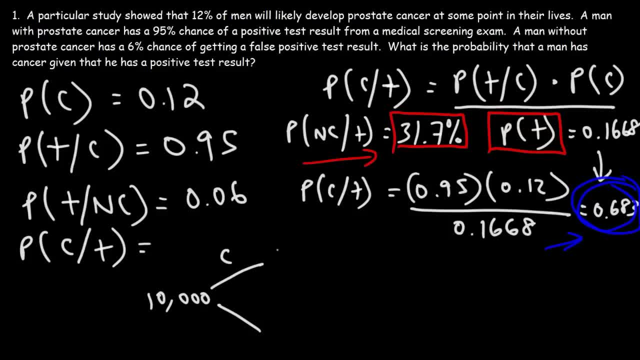 percentages: 10,000 times 0.12.. Is 1,200.. And the other 88% do not have cancer. So 10,000 times 0.88 is 8,800.. Now, of those who do have cancer, we know that 95% of them will get a positive test result. 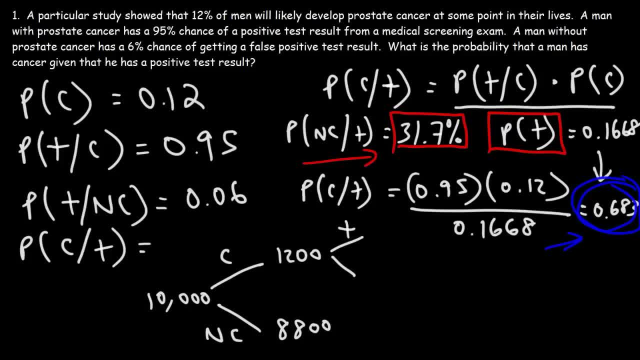 So 95% of 1,200, or 1,200 times 0.95,, that's 1,140.. So the other 5%, that's 1200 times 0.05, we'll get a negative test result, And so that's 60..